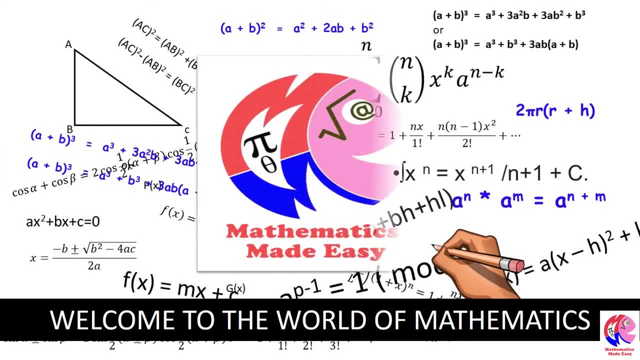 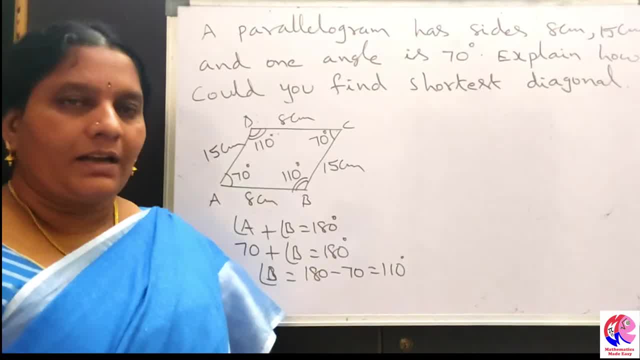 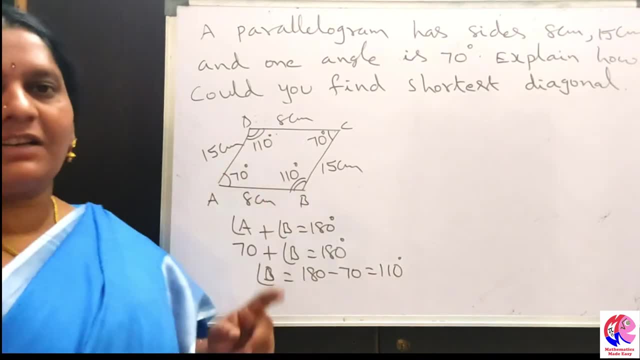 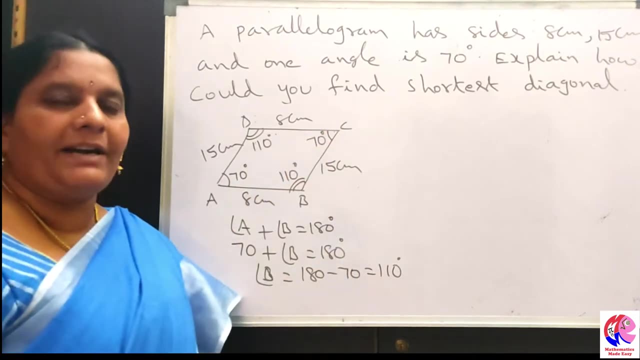 The sides of a parallelogram are 8 centimeter and 15 centimeter. Angles are 70 degrees and 110 degrees. By using this data we are going to find the diagonals of a parallelogram. Diagonal is nothing but the line segment joining the non-consecutive vertices. So in this parallelogram, 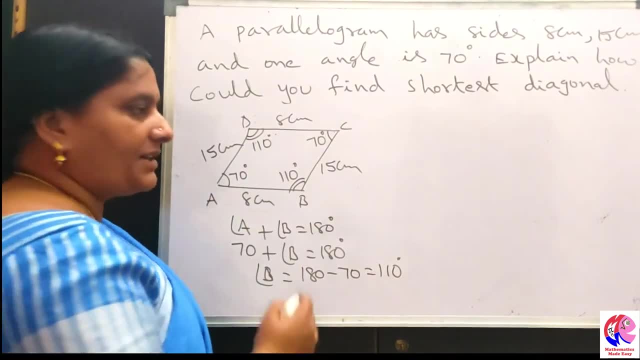 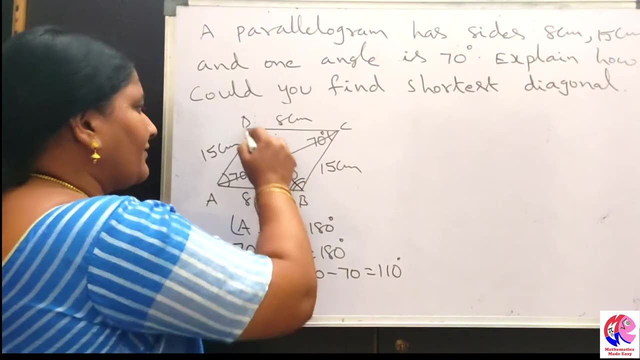 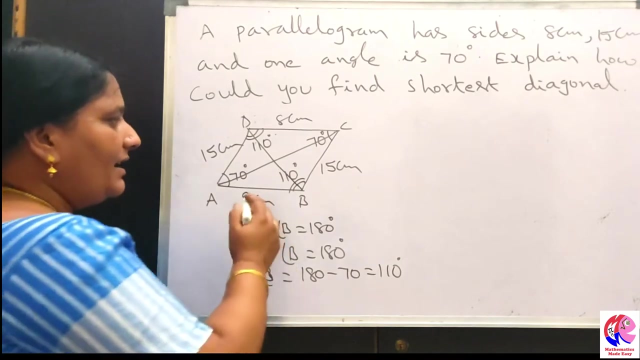 ABCD, A and C are called as non-consecutive vertices. So join AC, which is diagonal of the parallelogram. Similarly, BD is also one of the diagonals of the parallelogram. Let us find length of AC and length of BD. Now take the triangle ABC here separately. In this triangle ABC. 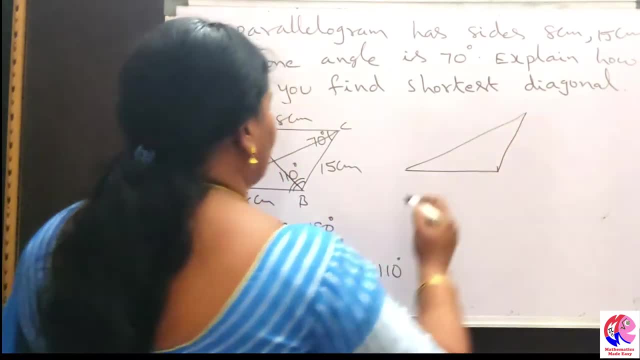 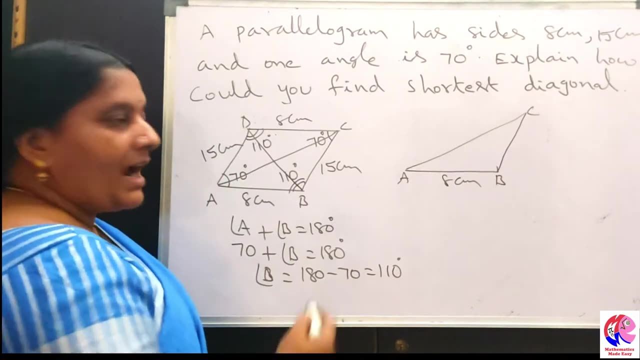 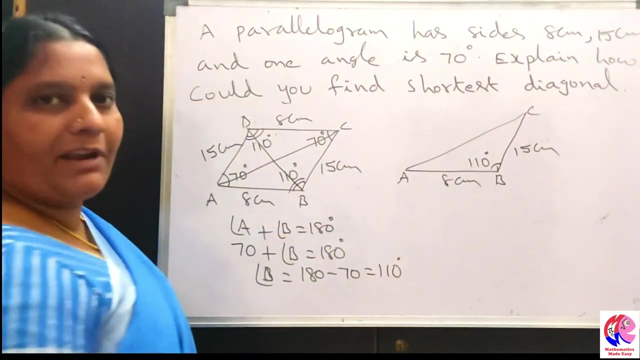 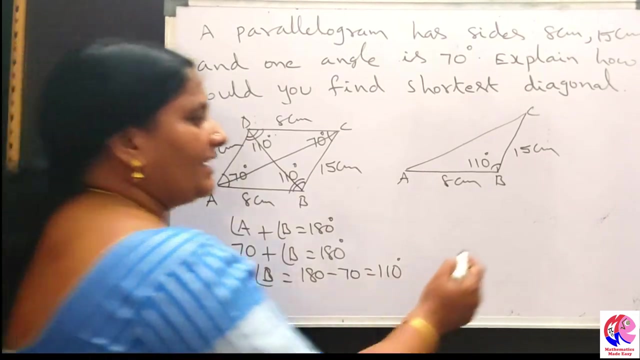 this is the triangle ABC we have. In this triangle ABC the measure of AB is 8 centimeter and BC length is equal to 15 centimeter. Angle B is equal to 110 degrees. Now we have to find the length of the diagonal AC. For finding this we are going to use cosine rule There in the 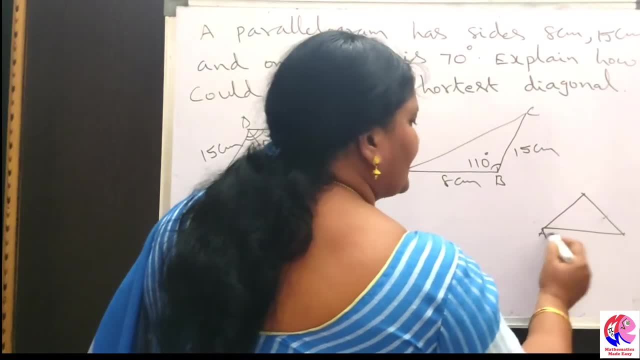 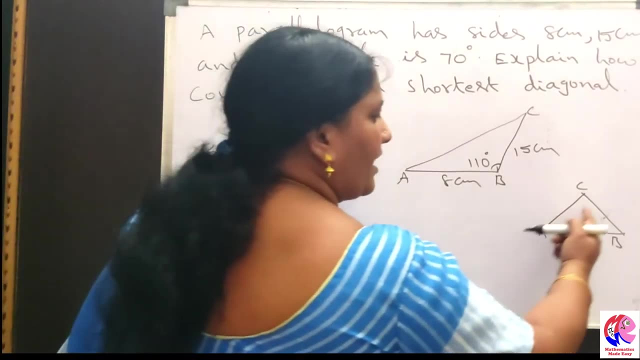 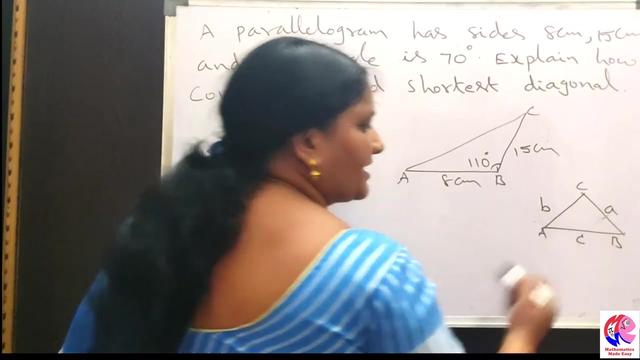 triangle. suppose a triangle ABC is given. In this triangle we have to find the length of the diagonal ABC. The sides we can represent by using lower case letters: Side opposite to vertex A is a small a. Side opposite to vertex B is a small b. Side opposite to vertex C is a small c. 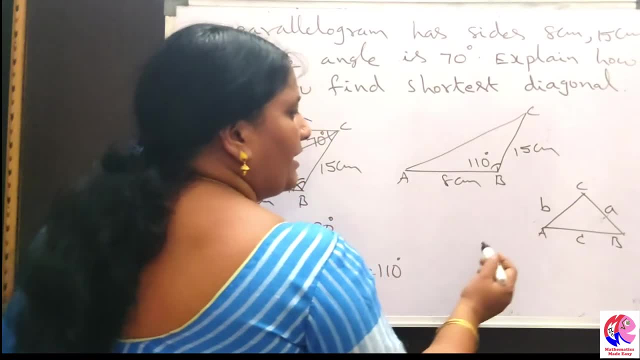 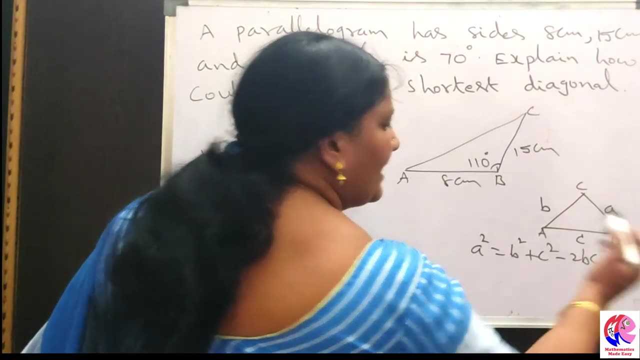 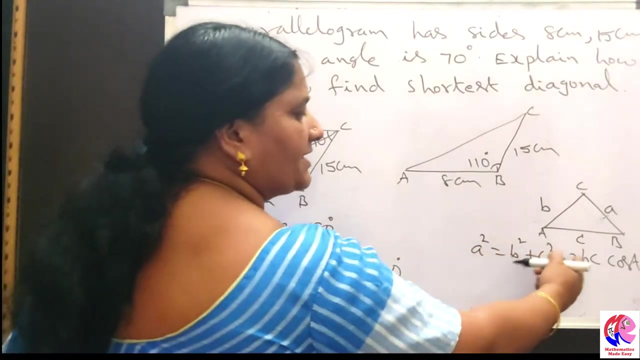 Then suppose we are going to find the measure of A. We can apply that A square is equal to B square plus C square minus 2 BC cos A. In this triangle ABC we can apply cosine rule: A square is equal to B square plus C square minus 2 BC cos A And B square is equal to. 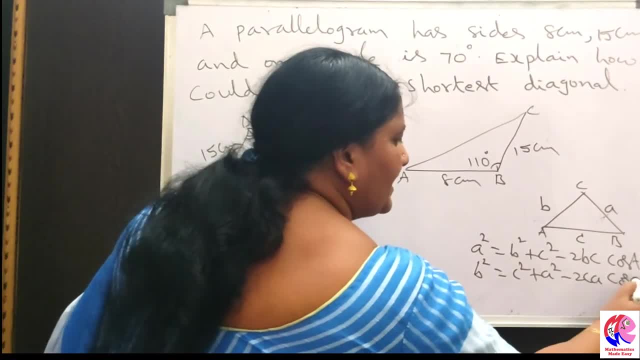 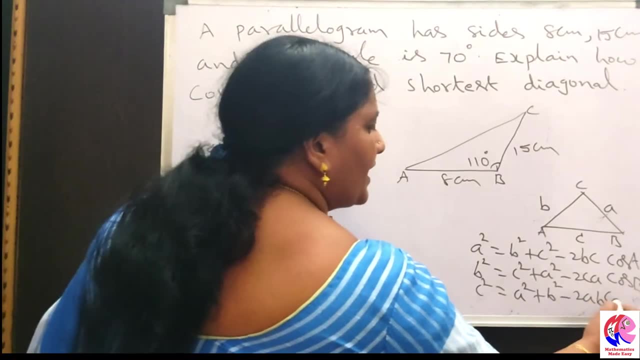 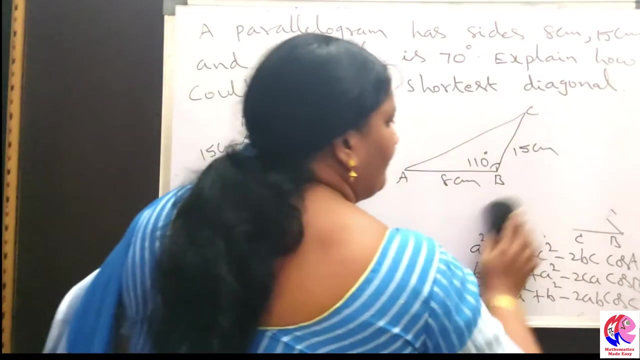 C square plus A square minus 2 CA cos B. C square is equal to A square plus B square minus 2 AB cos C. So this is called cosine rule. Now coming to the triangle ABC. In this triangle ABC we are going to find the measure of AC. 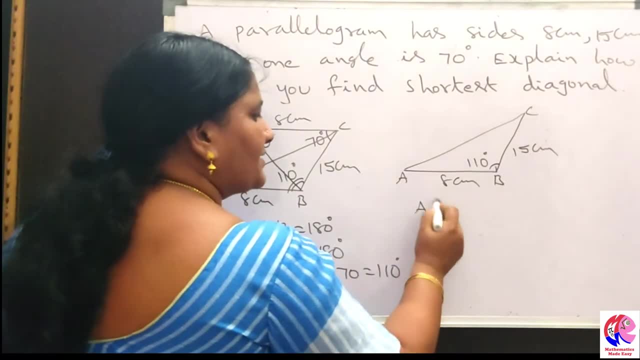 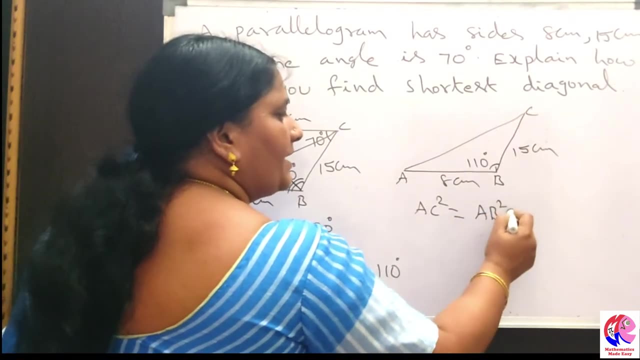 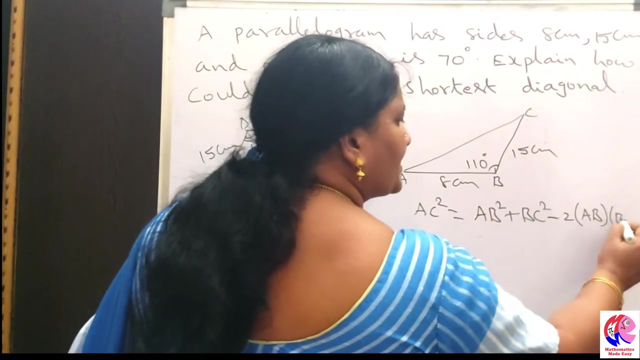 So apply cosine rule. So B is equal to A b, B is equal to A c. So let usrants F equals like cosine rule. a c square is equal to a c square is equal to a b square plus b c square. a, b square plus b c square minus 2 into a b, into b c, into cos b, which is equal to the measure of. 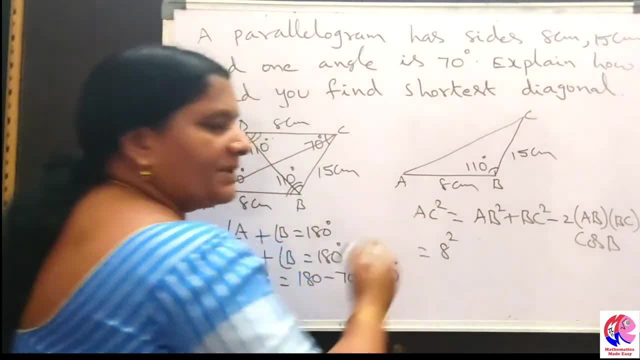 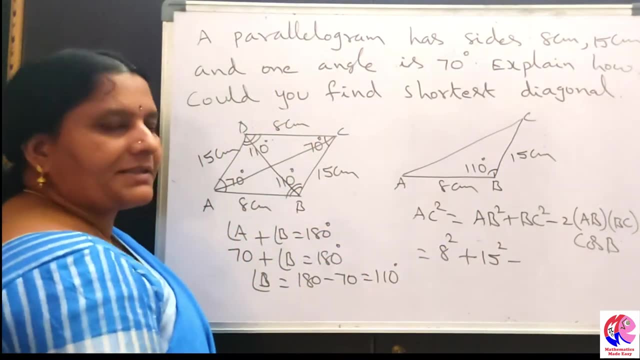 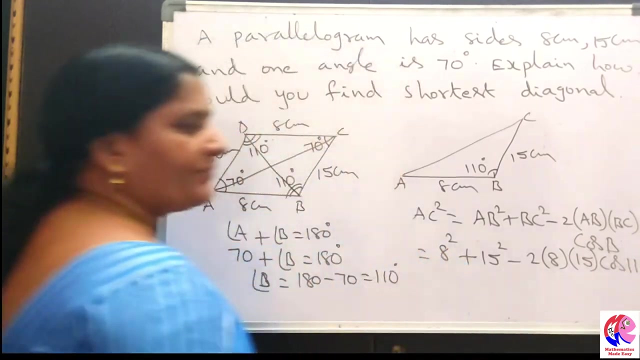 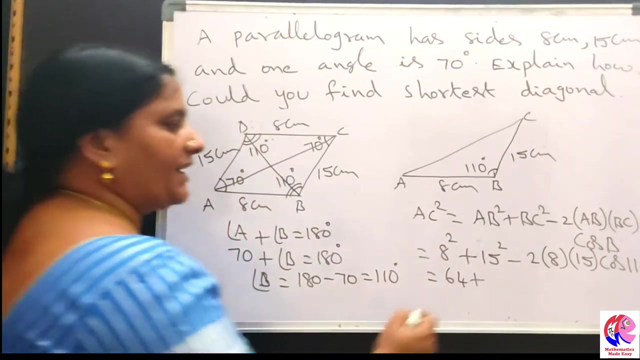 a, b square. i mean a, b is 8. so a- b square is 8 square plus b. c square is 15 square minus 2 into 8, into 15, cos 110 degrees, cos 110 degrees, then 8 square is 64 plus 15 square is 225 minus. 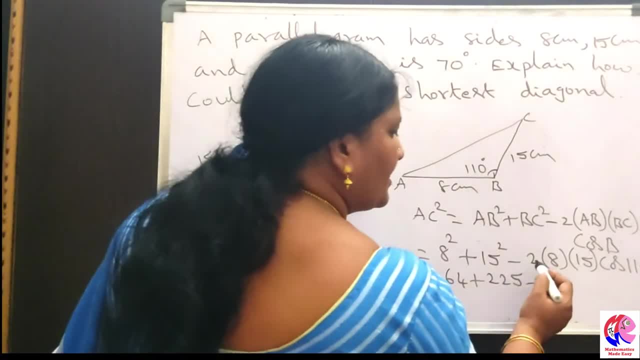 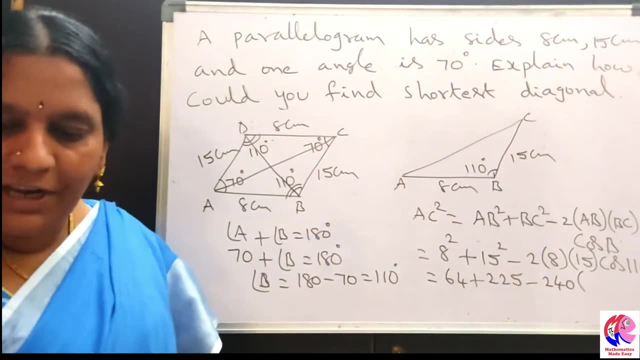 2 into 8 into 15. 2 into 8 into 15. 2 into 8 into 15. it is 2 into 15, is 30, 30 into 8, is 240 into cos 110 degrees. we can find cos 110 degrees. 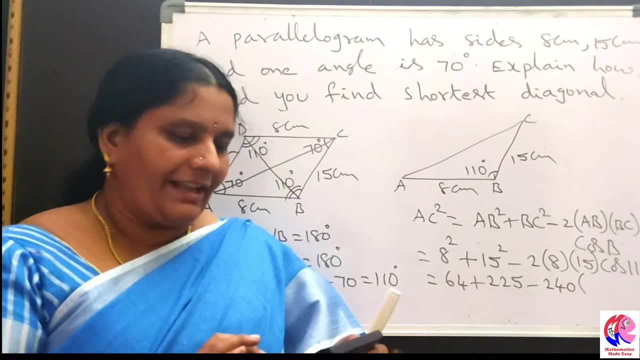 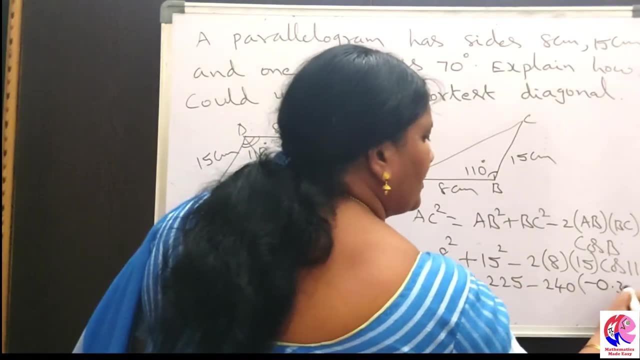 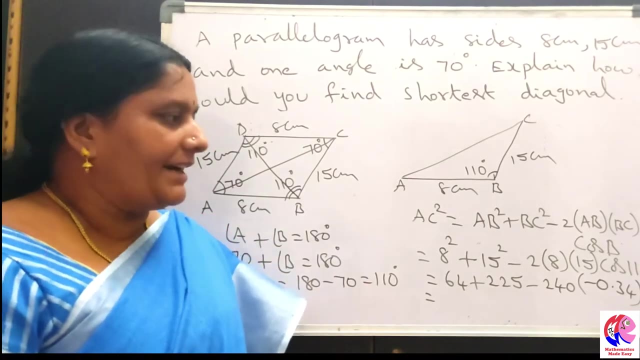 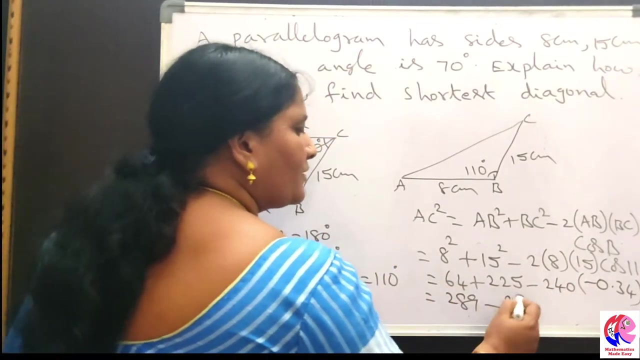 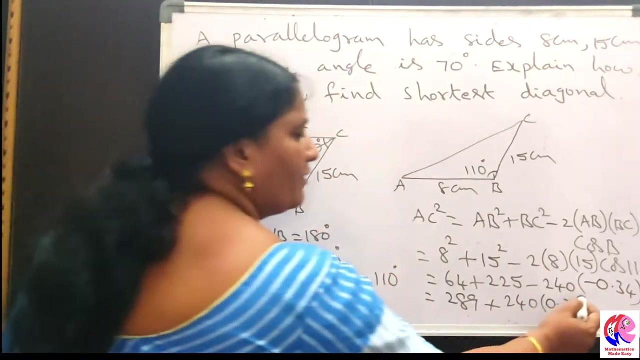 by using calculator. so cos 110 degrees value is equal to minus 0.34. it is a minus 0.34 because cos 110 degrees is in the second quadrant. in second quadrant cos is negative. so cos 110 degrees value is a minus 0.34. now it becomes a 289. minus 240. into minus, into minus becomes a plus 0.34. now i will calculate. 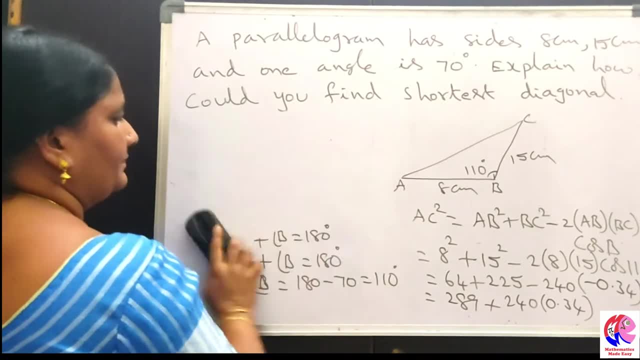 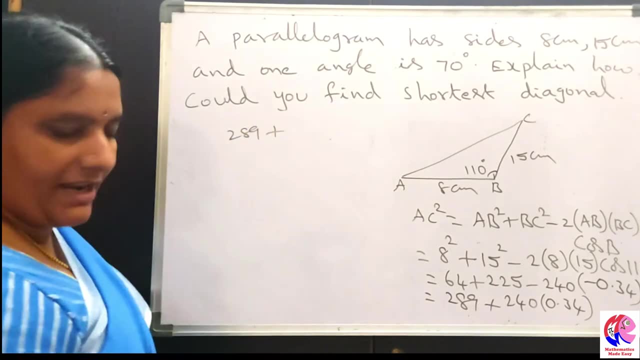 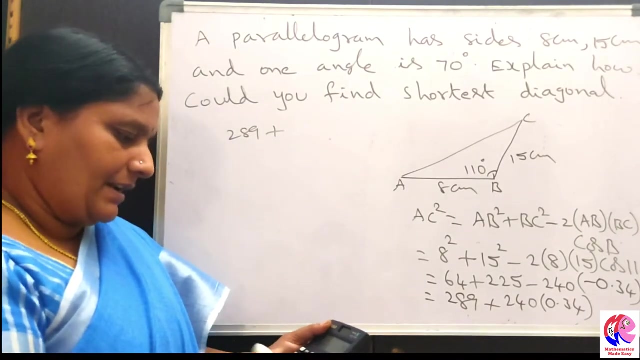 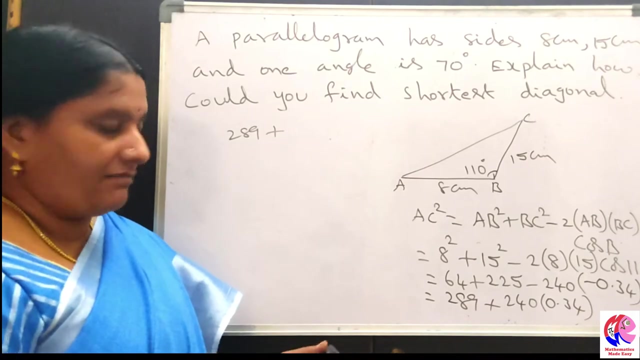 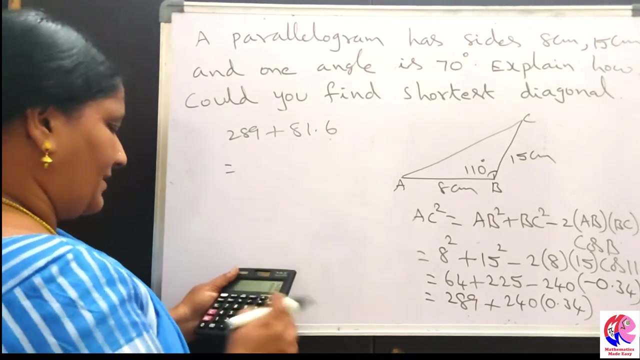 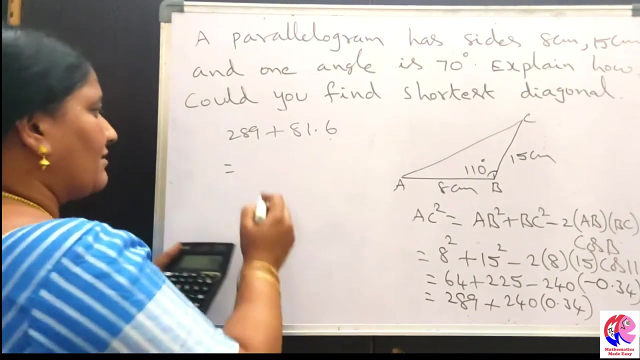 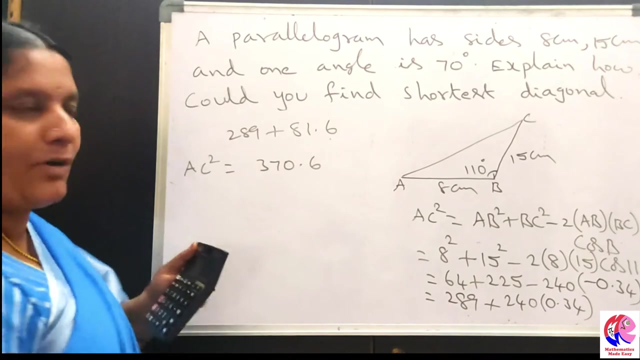 this value. here this becomes a 289. 289 plus 240 into 0.34. 240 into 0.34 value is equal to 81.6. this becomes 289 plus 81.6. we can find: here it is 289, which is equal to 370.6. so here a c square is equal to 370.6. measure of a b square is equal to. 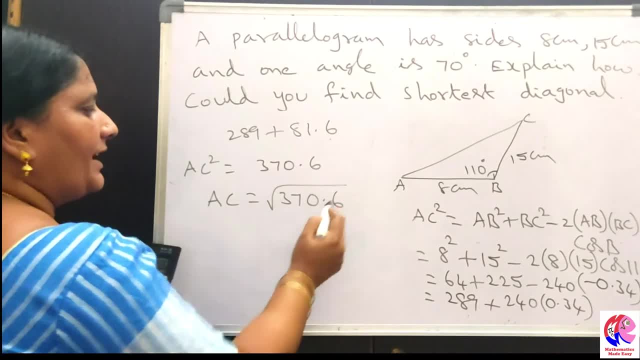 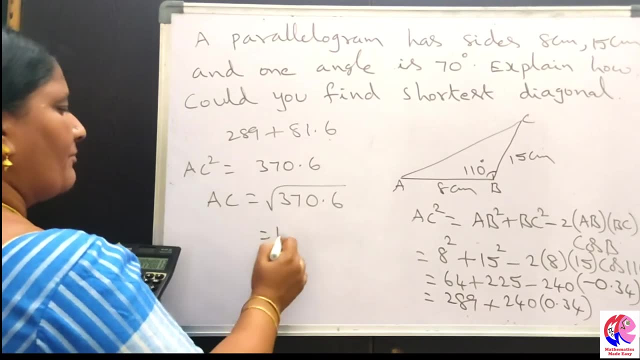 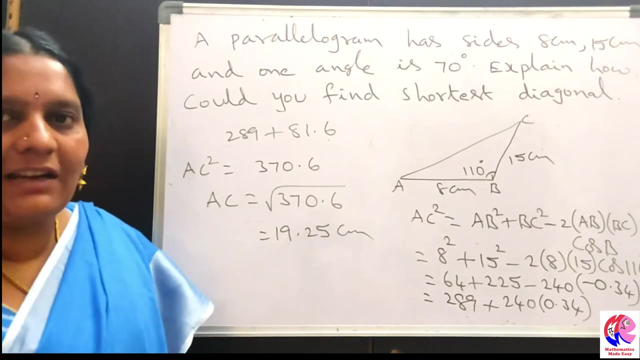 root of a c is equal to root of 370.6. now square root of 370.6 is equal to 19.25 centimeter. this is 19.25 centimeter length of the diagonal a c. we can find the diagonal b d also, so for 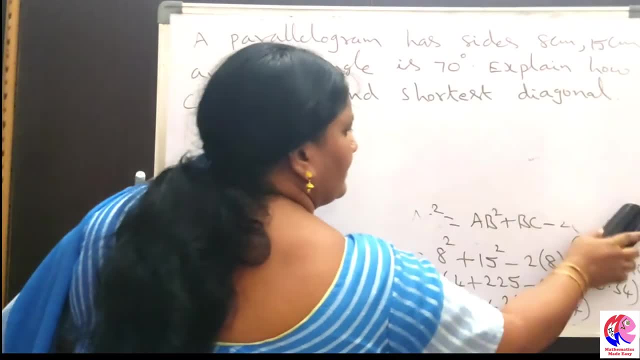 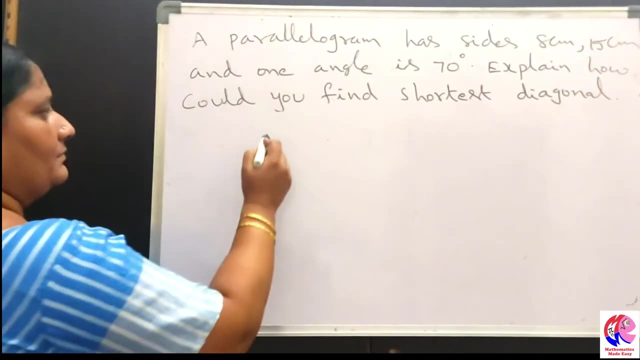 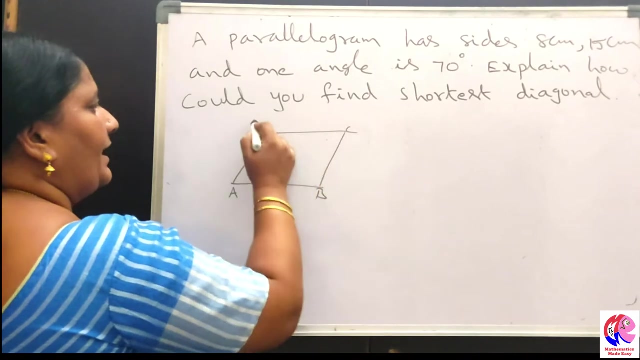 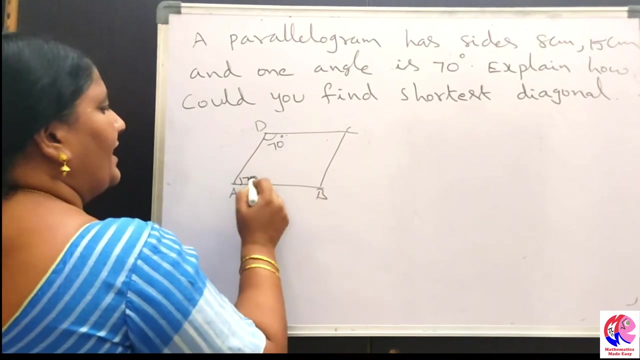 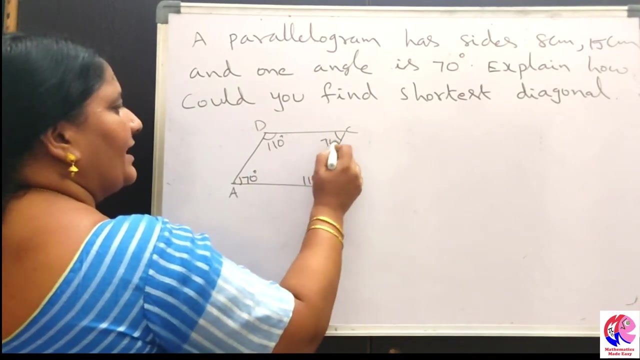 finding the diagonal b d, let us find the measure of a c square. we can find the diagonal b d also. we have taken in this parallelogram a, b, c, d. here it is 70 degrees. now this is 70. this is 110 degrees. here it is 110. this is 70 degrees. for finding the measure of b d, let us take the triangle. 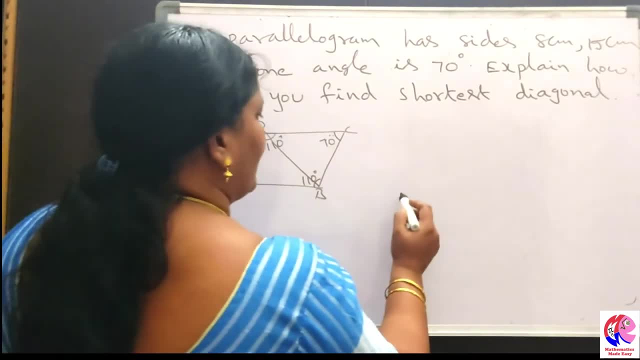 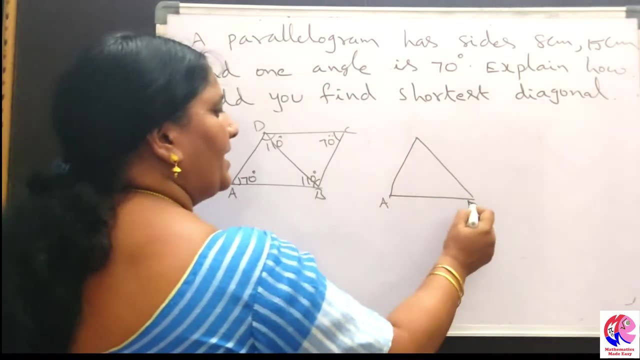 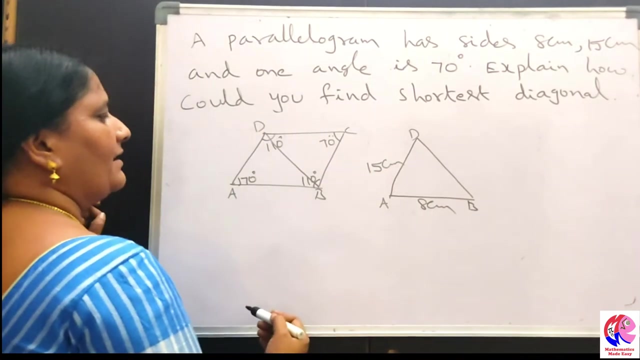 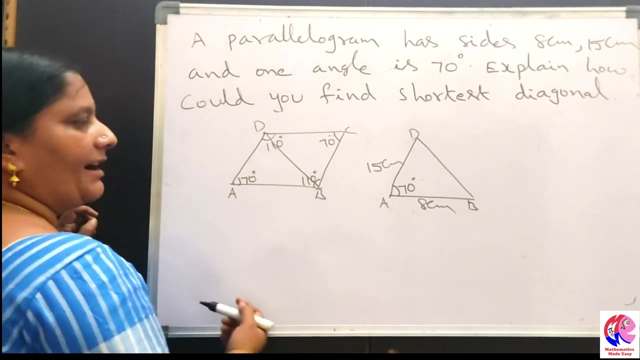 a, b d in this triangle a- b d. our triangle a- b d will be like this: a- b d, the measure of a, b is 8 centimeter and a- d is 15 centimeter and angular measure is equal to 70 degrees. now we have to find the diagonal b d of the quadrilateral, again by using cosine rule. 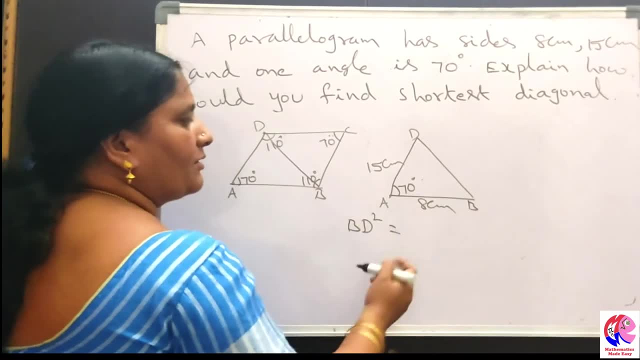 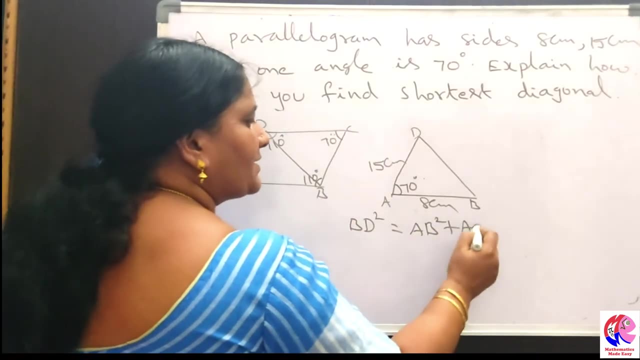 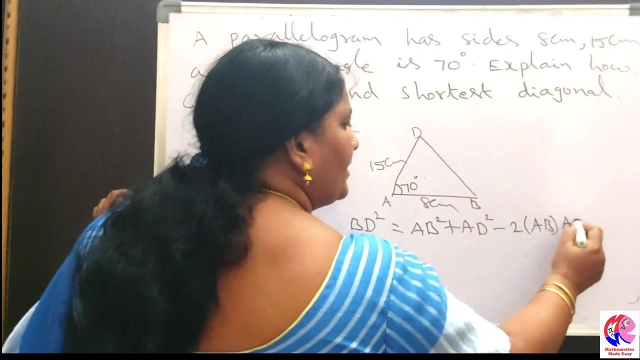 so b d square is equal to 70 degrees. so we have to find the diagonal b d of the quadrilateral bd square is equal to ab square plus ad square, ab square plus ad square minus 2 into ab, into ad, into cos, a cosine rule. 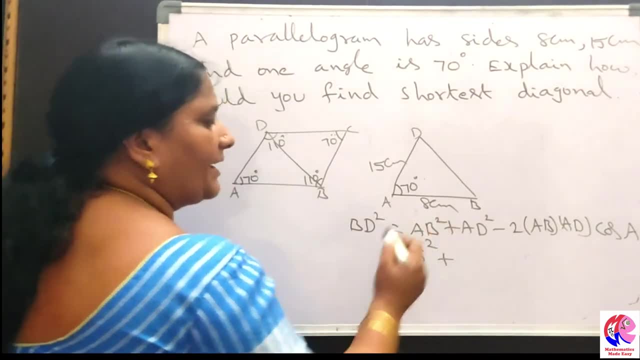 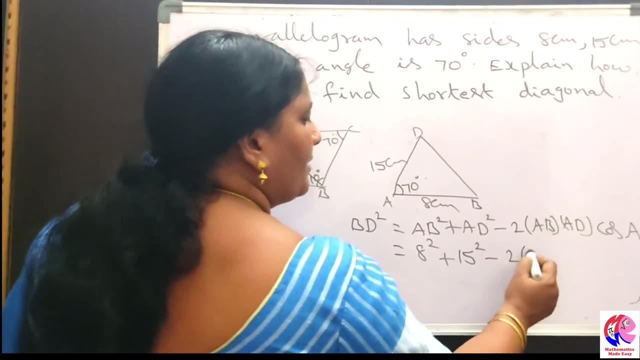 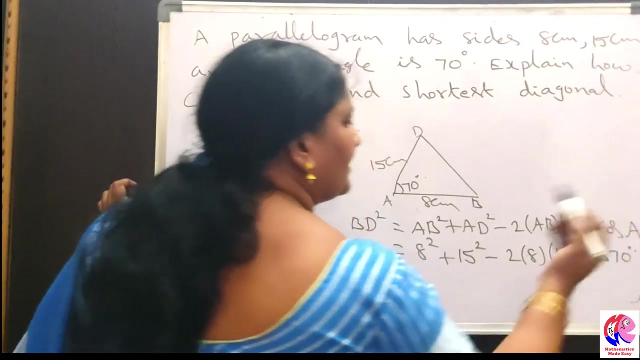 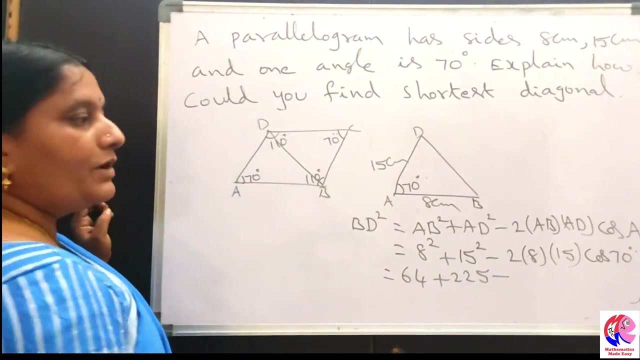 So ab square is 8 square plus ad square, which is equal to 15. square minus 2 into ab is 8 into ad is 15 into cos 70 degrees. Now it is 64 plus 15. square is 225 minus 2 into 8 into 15..